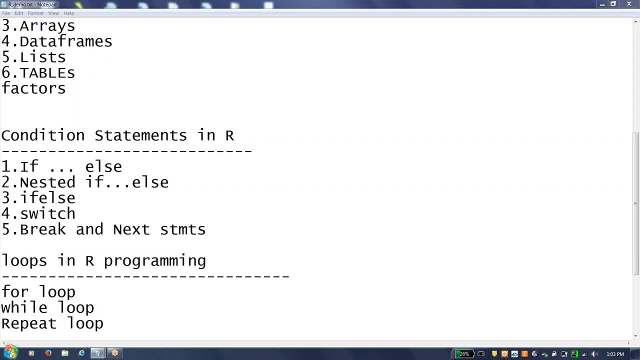 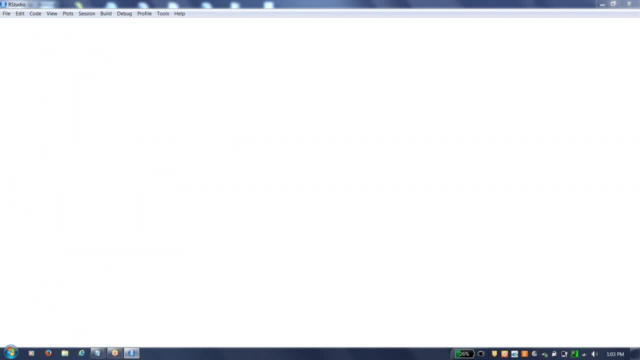 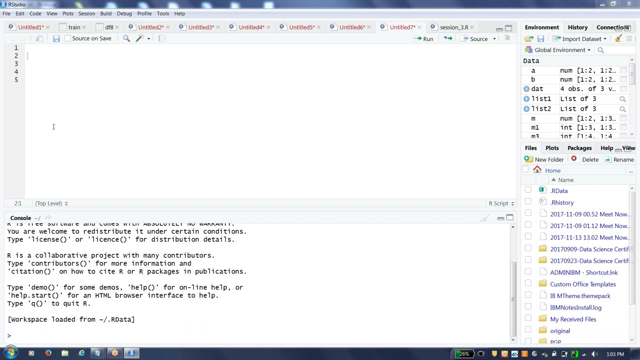 going to execute the statements in else part. So let me show you an example here in R studio. So I am going to launch R studio here. So, ok, fine, Here I have R studio. So let me create a variable like: so age, because age I can say. 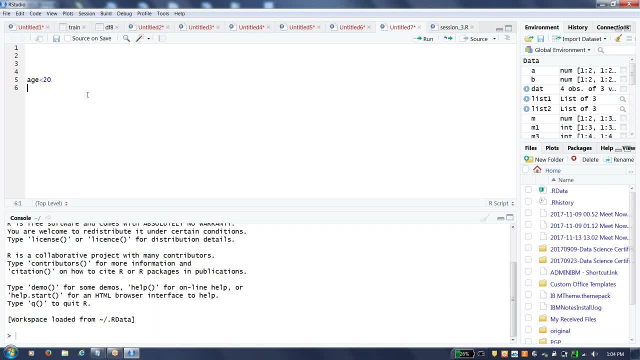 I am assigning age value with 20.. And my conditional statement here is like: suppose, if age greater than 18, 18.. So what I want to write is: if age greater than 18, 18.. So I am going to print, print, pri and print within quotes major: If age greater than 18,. 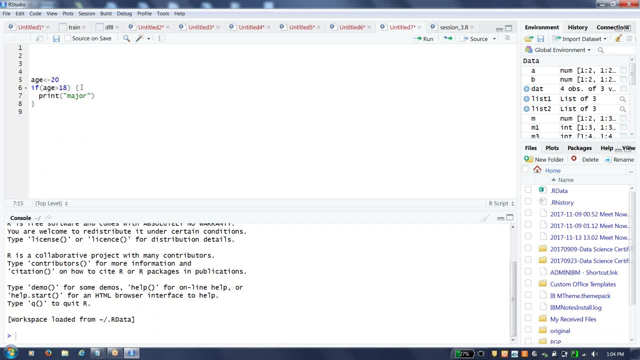 obviously we are going to tell major. So here the thing: when you write R programming. so this syntax is like this one. So if age greater than 18, you should open curly braces here on the same line So that it will expect there are no variables. So if age greater than 18, you should open 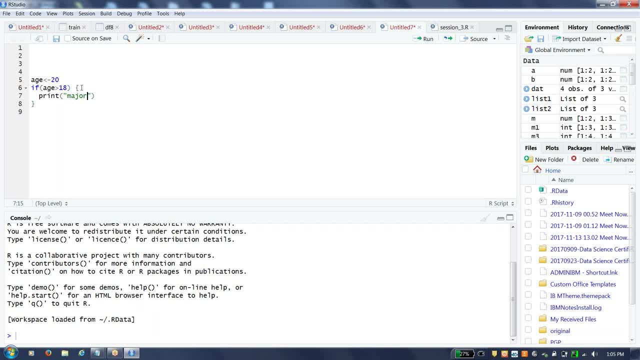 curly braces here on the same line, So that it will expect there are no variables. So that it will expect there are no variables So that it will be any code in the next line. So if you enter the this, it will be problematic. Otherwise you need to add a plus symbol that 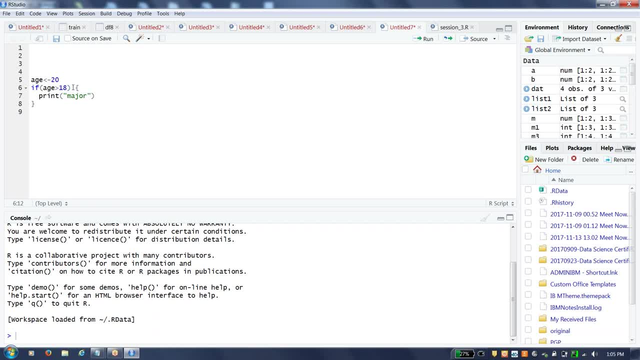 is another thing that I'm going to explain. next next two videos. So always keep like this, only if age greater than 18, you need to keep it this curly, press open, curly braces in the same name. then you make your write, you will print statements. 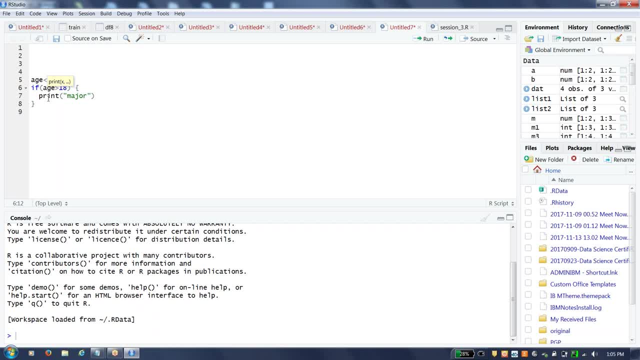 Or whatever the hop you would like to or whatever the character you would like to do in this area. you do it and then close the curly braces and also else. statement should start in the same line wherever. if statement curly braces, close it else and then you open your curly braces for else and statements on the same line and then 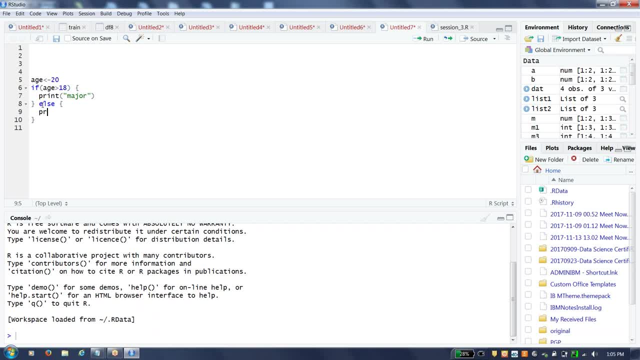 so what we are trying to do is, if not, here I empty print. what I am going to print is say it is minor, age is greater than 18, I am going to print major. if not, it is going to come into that else loop and it else else statement. then it will. 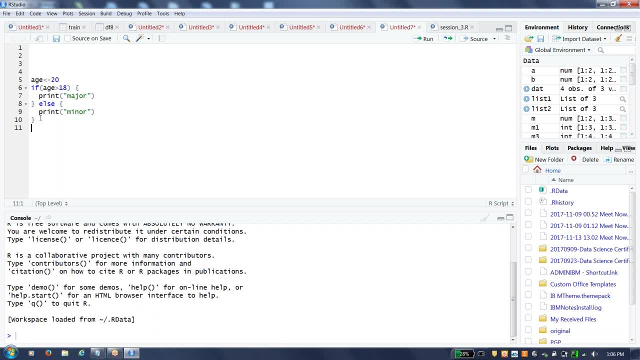 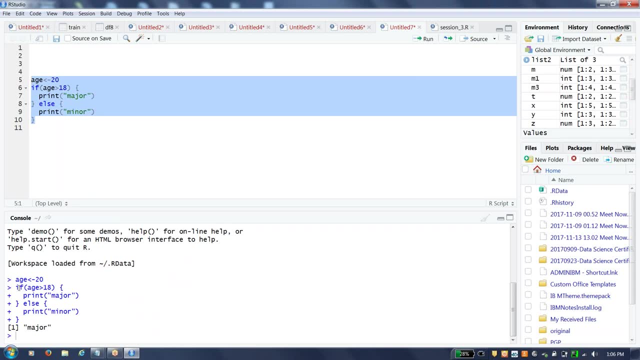 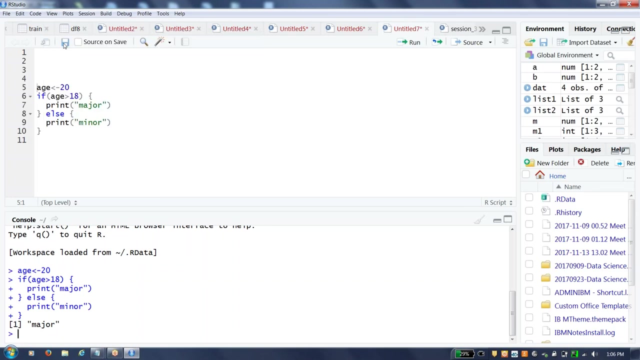 print minor. okay, so let me run this script and see what it is going to give me. so this script is run here and and, as you can see, the result is major. so maybe let me zoom this some more, maybe, but now it is not visible, but clear. we do one more time. 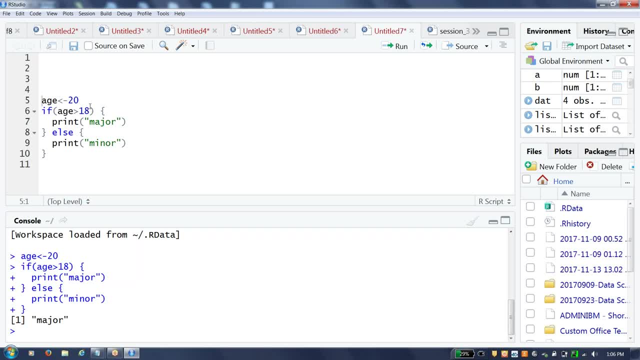 yeah, fine, so this is my script. so I provided here some input for age variable and that age variable and checking whether that value is greater than 18 or not. yeah, a greater than 18 means I am going to exclude my print statement major if not. so what we are just going to do is create an age in which, if we rồi, 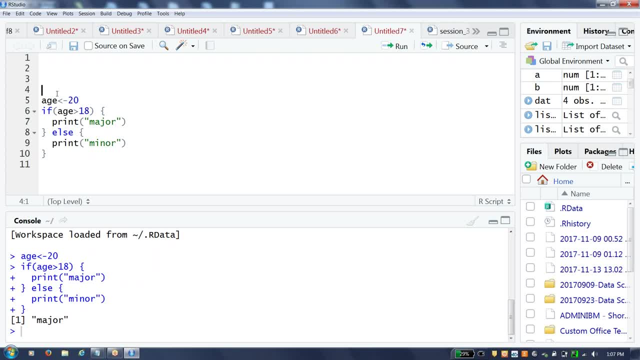 do not tell me without telling you that we are going to write. I just make sure you know the statement. Okay, so now, if it is, if it is greater than 18 gr, i am going to execute my print statement. major, if not else case mean I am going to print a manual statement. if not else case mean, I am going to print a abdominal statement, so this is how this its else is what is going to work, so let me write. if this else this is what is going to work, so let me write so. and one more thing: R Programming the command like this, so you can use this symbol and write if an statement is required. 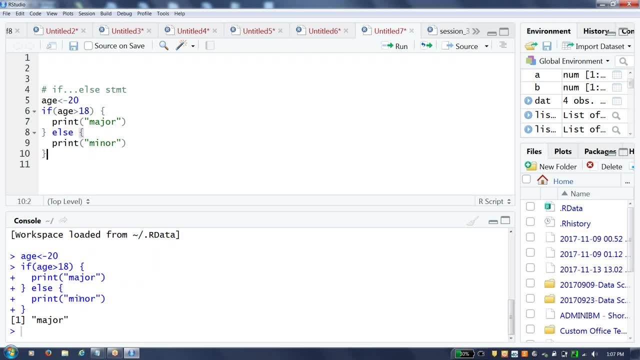 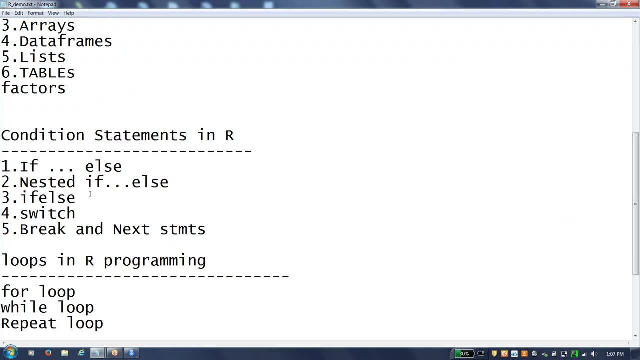 statement: okay, this is for if else statement. okay, uh, coming to the next one is nested if else. so how this nested if else works it. so it's nothing but an if inside another if statement. so like it's. it's like long, uh uh, procedure means a number of if statement. like more than uh, one condition: we are checking, then we are going to. 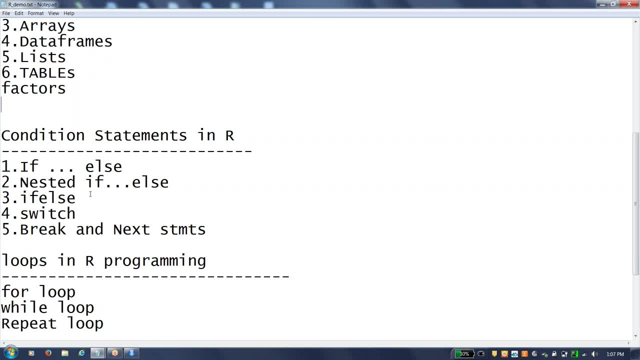 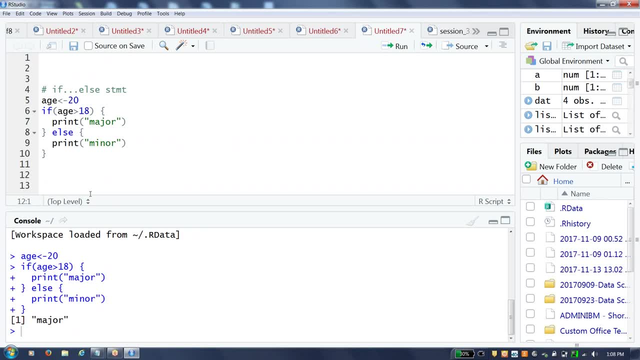 use this: uh, nested if statement, so for this also. let me take you, show you one example for this. so let me write here: comment, what is comment? so nested if statement, okay, so for this. so i'm going to write another example. any, any simple example you can write so simply. 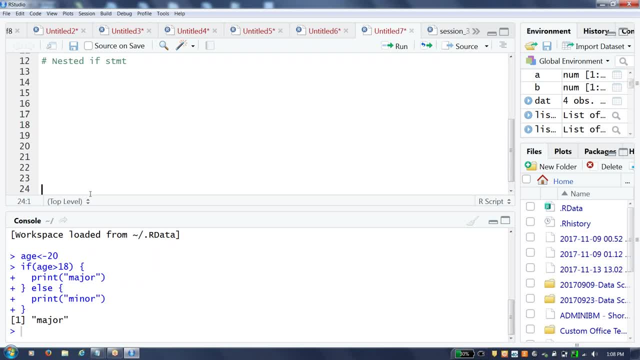 i want to check whether a number is a positive number or it's a negative number, i'll say zero. so there are more than uh two possibilities. then i'm going for nested. if so, what? i'm going to take it any variable, i'm taking x, so i'm going to assign a value, 10 suppose. so what, i'm going to. 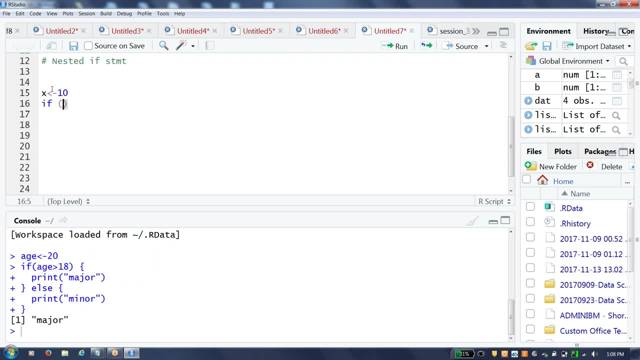 check is: if x, x less than zero, what i'm going to do is i'm going to print. i'm going to print negative number, so similarly my else, if else statement, el else else, if, if, if x greater than zero, then what i'm going to do is print: 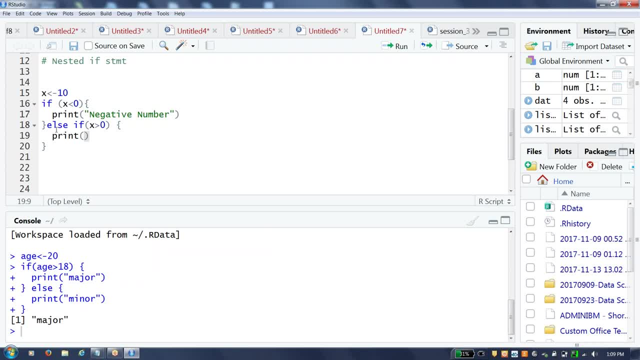 positive state was the number okay. so these are the two conditions. of course, if not these two conditions, there may be another condition which is else part that i'm going to write else else i'm going to print zero okay. so let me run the script okay and see. so if i provide 10, it has given me positive number. 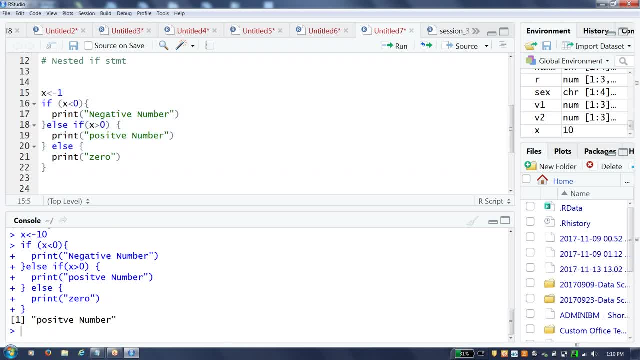 if i provide 10, it has given me positive number. if i provide 10, it has given me positive number. is the result if i provide me some some negative number and run the script. so it is giving me negative number. and let me try the other possibility also. 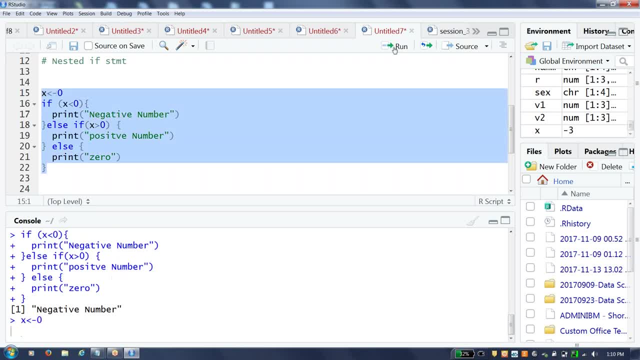 so it is giving me negative number, and let me try the other possibility also. so it is giving me negative number and let me try the other possibility also: zero. if i provide zero, if i provide zero, if i provide, it is going to run and give me the result. 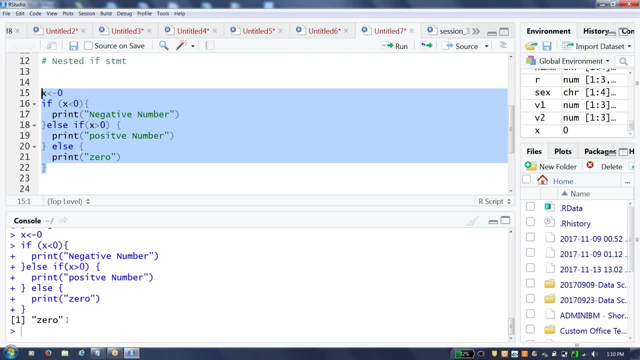 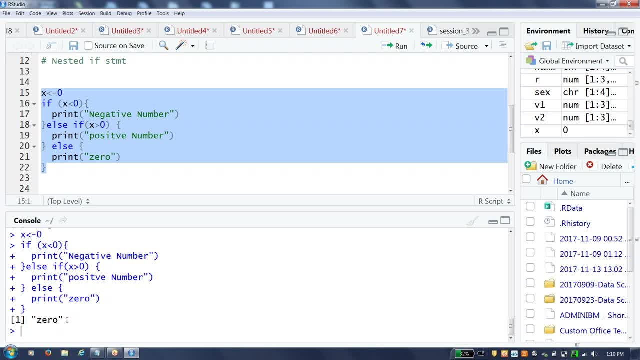 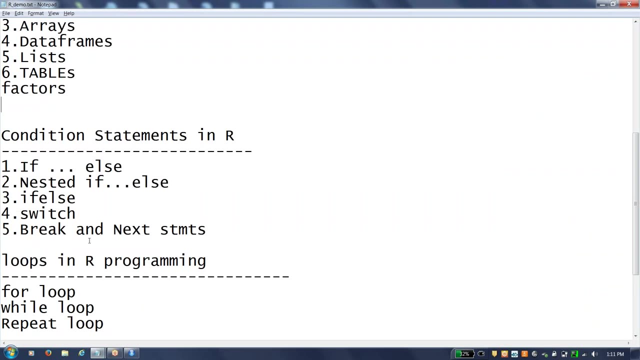 two possibilities, two possible ways. then we are going to use this nested if statement. so, more than two possible ways. then we are going to use this nested statement. okay then then let me cover if-else statement. it's like: suppose I have multiple values. it's a vector, set of elements in a vector. that vector, if I want to use it. 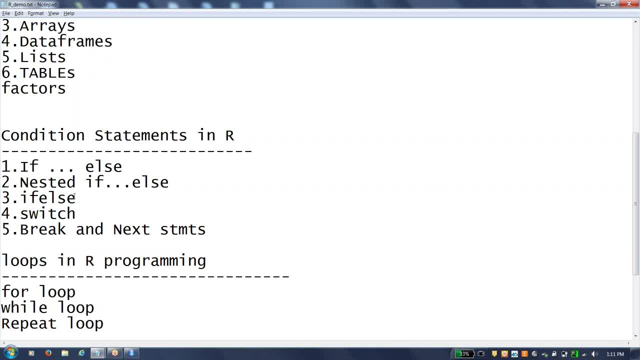 in a if statement and want to check all the elements in that if condition and if I want to give a result of that. okay, if that condition is true, what I want to do. if that condition is false, what I would like to do. so those, those things I can. 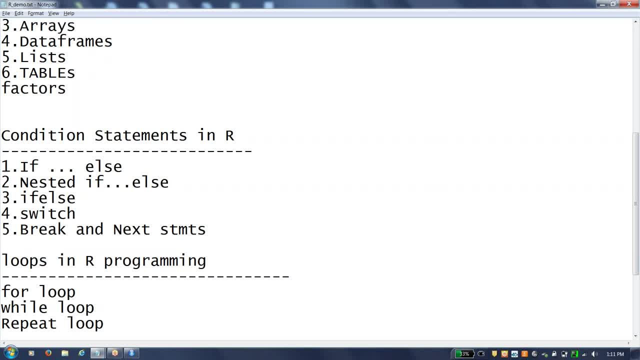 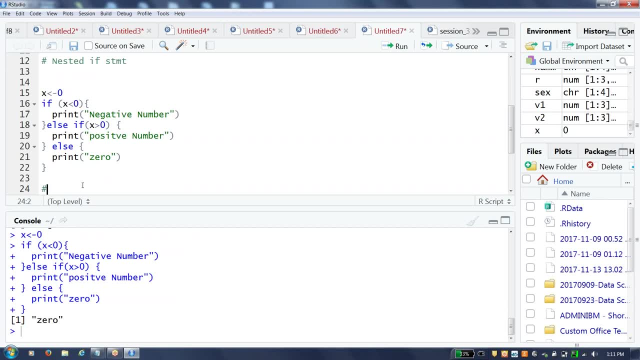 get it are done in using if-else statement. so suppose, so you a third statement. I can say here if-else statement for this simple syntax. one line, one line syntax. so suppose I have a vector a which is having some one, four, six, four, seven, eight and nine, okay, 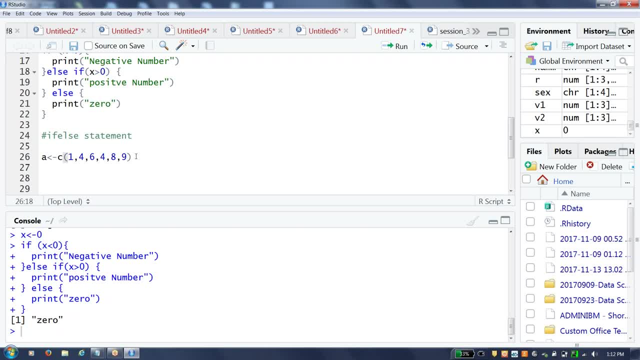 so all this set of numbers I have, okay. so what I want to see is if-else this set of elements in a are even numbers, are odd numbers? that I want to find out. it's not one element, it's, it's a set of elements that I want to. 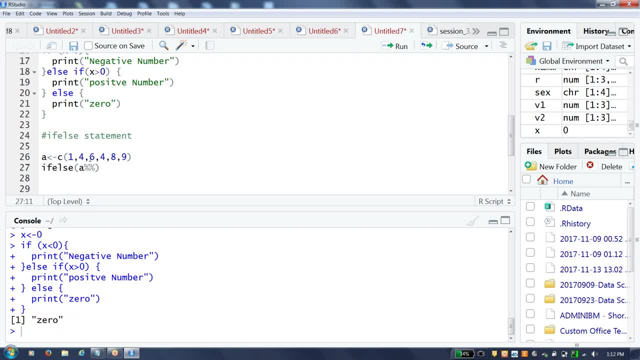 check, and also in one line statement I want to check: if a percentile to a word less two equal to equal to zero, then even else, are so always this character things, character strings? I need to put it in quotes. so then let me run this script. okay, so what is missing is so always one thing we should remember in our studio. 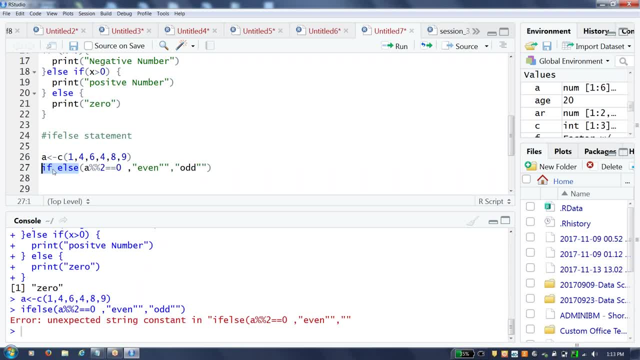 if. if it is a keyword, like else, if switch. if it is a keyword, it should be in blue color. so if I remove the space, it's not reading as a keyword. it's not if it's actually fell statement. it is treating us like a, some kind of a variable or some kind of text like that is stating so it's not a. 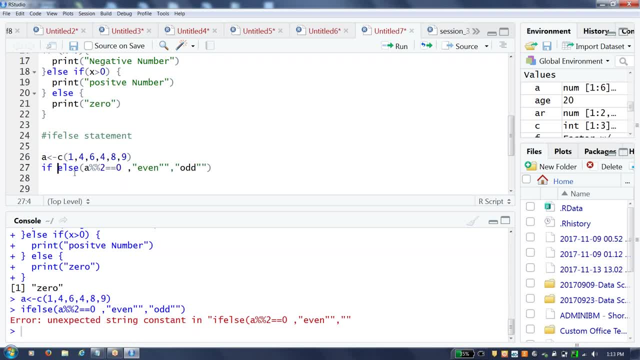 keyword. so if you space it, if space else is the correct statement, not if else, maybe you're wrong here. okay, so if else a percentile to a model is two equal to zero, then even otherwise it's odd. so then let me try one more time now. okay, again I. 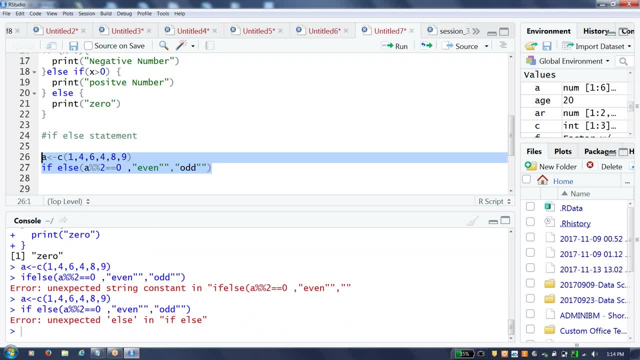 will run this script here. and what error. so sorry, I was wrong again. so it's if we thought space. only I thought here double quotes are there because of that it was giving, but I wrongly interpreted and the reason so if else here, if I run this script, I am going. 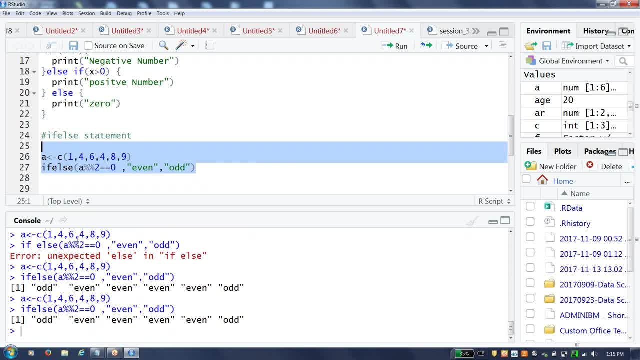 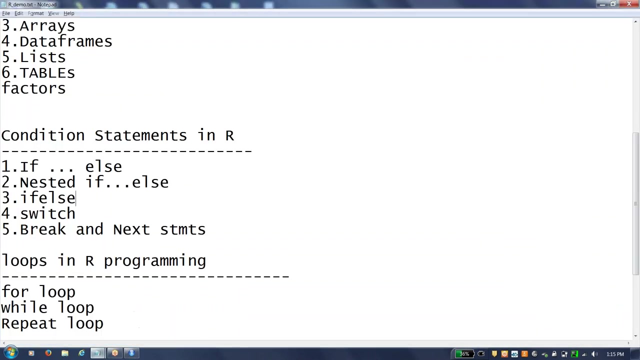 to get the result here like this: okay, odd first, one is odd, one is odd, four is even, six is even, 4 is even. again, 8 is even and 9 is odd. so I'm going to get the result like this: so this is the functionality of if else statement. so now, moving on to the next one. 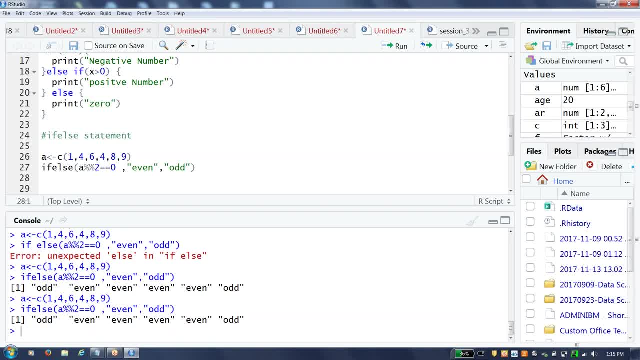 switch statement. which statement? this is also a very simple one. okay, how it works is: it will consider: first element of this switch is our input arrow. okay, how it works is: it will consider: first element of this switch is our input arrow parameter variable first variable, then that it is going to consider the corresponding. 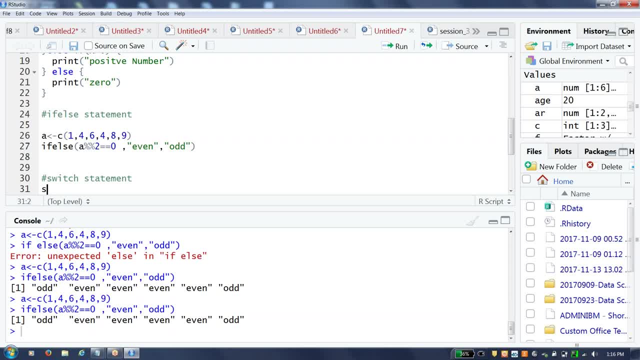 result set. so suppose if i have, if i see example like, then we can get clear picture which of suppose two comma say apple ball cat. so if i run this script, switch, switch statement, what is going to give me is switch that the condition. here what we are going to get is the condition. 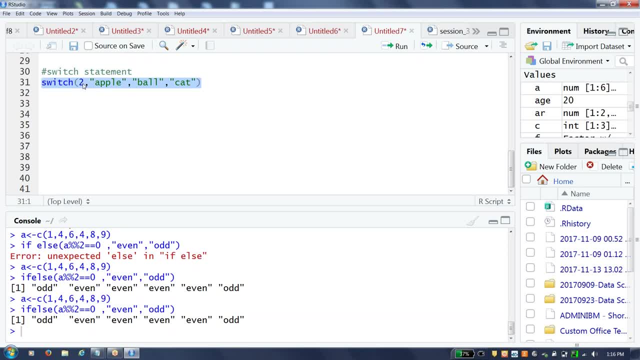 statement. so what is the second uh element in this out of these three elements is apple ball. cat is a ball, so if i run this, it is going to give me the result as ball. so like this it will work. so otherwise i can say another example. simply, i define a variable, a, which is, which is having values of two, and then 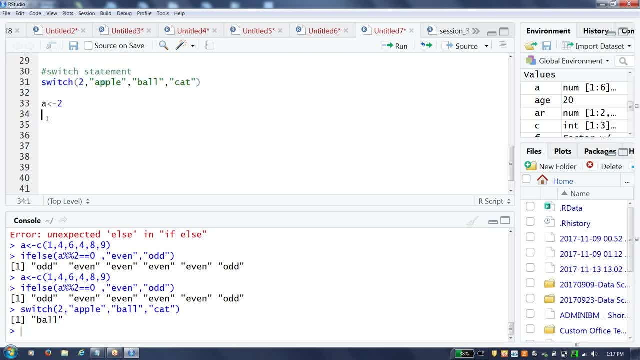 i can have the same switch statement. i can use it here. or i can pass this a as a value, so now i can run this. two scripts to run two statements. so so here also i can get two. i can change it to one. so now again i run. so so a value is one, so one is nothing but apple here. so it will give me a result. as apple. so now i can run this. two scripts to run two statements, so here also i can get two. i can change it to one, so now again i run. so so a value is one, so one is nothing but apple here. so it will give me a result as apple. so it will give me a result as apple. 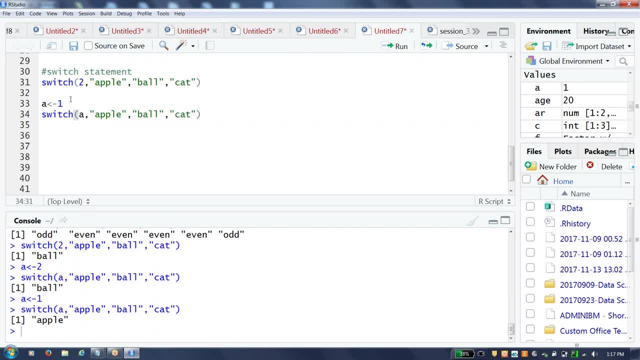 suppose if I give here same thing, what I'm going to get for 4, so if I give for, what I will get is no output, because we don't have any. we don't have any fourth element here, so one, two, three only we have. so for we don't have, it will give. 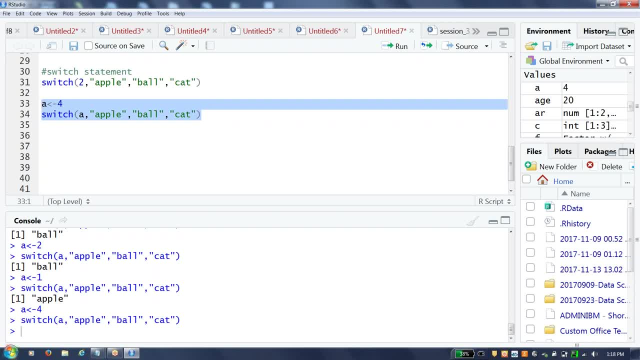 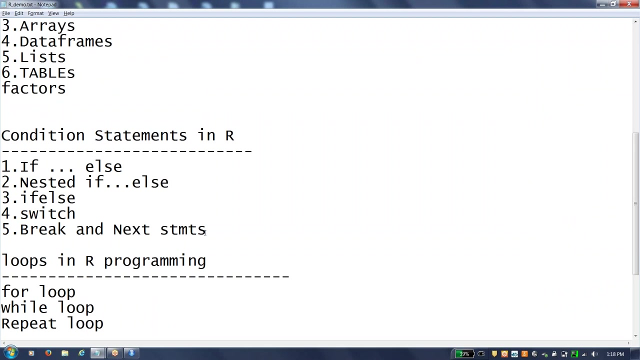 no output. so simply switch statement run and it is coming to coming back to again consume corresponding cursor. again not no output here. so this is how switch statement works. then let me move on to the next thing, which is break and next statements. how this break and next statement works, let me show you so okay. 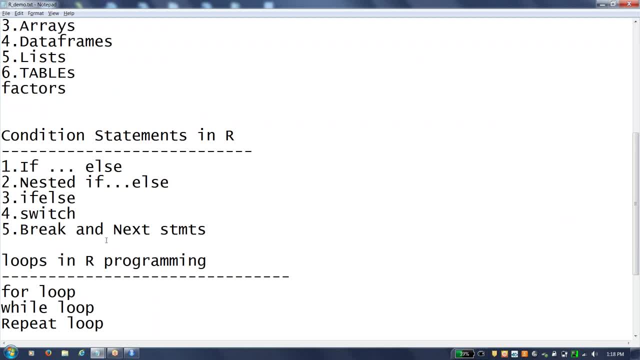 before this, before this. so I need to explain this break and next statements along with. So let me explain for loop, then I can go with that break and next statement. so loops in our programming, for loop, while loop and repeat loop, so for loop, we it is very simple: in our programming we can: 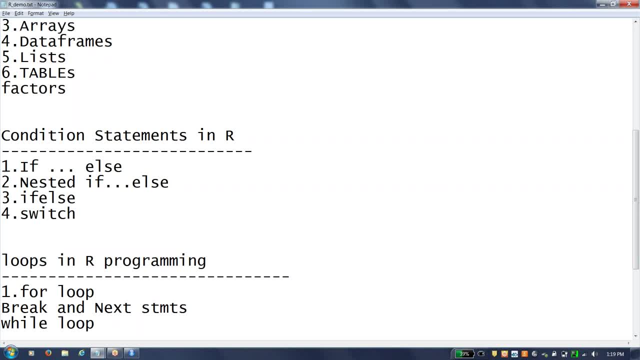 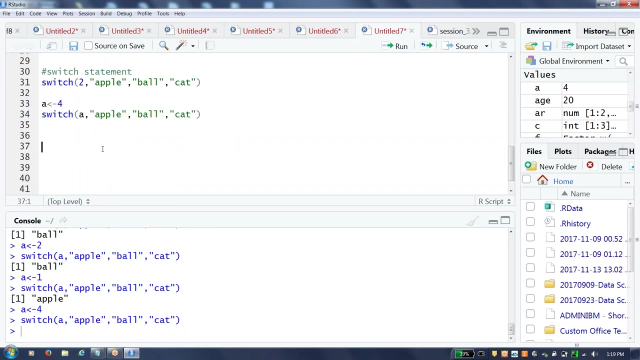 repeat the loop n number of times. how many number of times you want to repeat those many number of times? we can simply repeat, but in, in there is no implicit condition. in for loop there is no implicit condition. so only we can repeat the loops. there is no condition here. so let me show you an example for that as well. so example here: 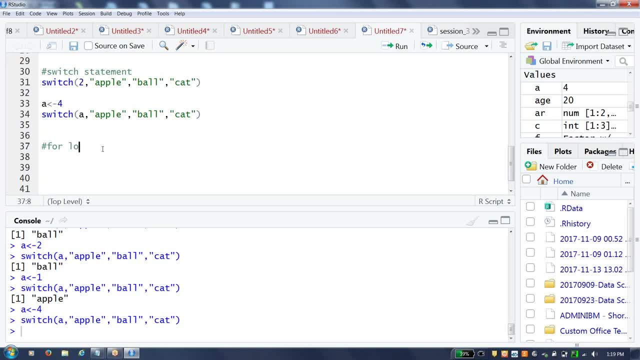 loops. so if I have a vector, if I create a vector which has some 1, 2, 3, 4, 5, 5 elements, so which which I want to print, so for V a L in vector V C, then what I am try print. so here a statement, any statement you can write. 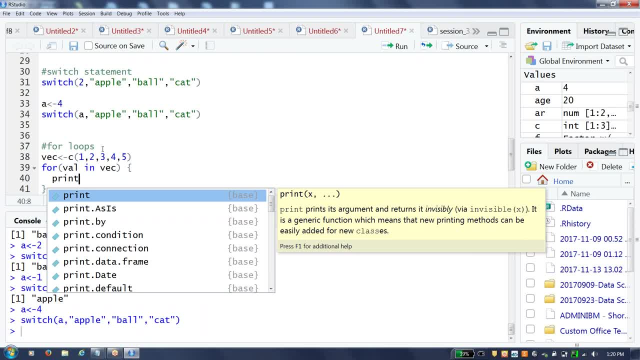 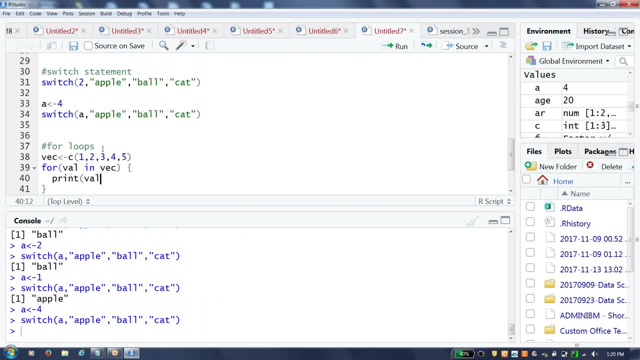 any manipulation and with this actor elements we can do over to here. I just simple example. I just I would like to just print. I'm just printing vector V, easy and pretty vector. so what I'm going to get is simple vector values five times okay, so it's, it's like vector is having five elements. okay, sorry, vector is having. 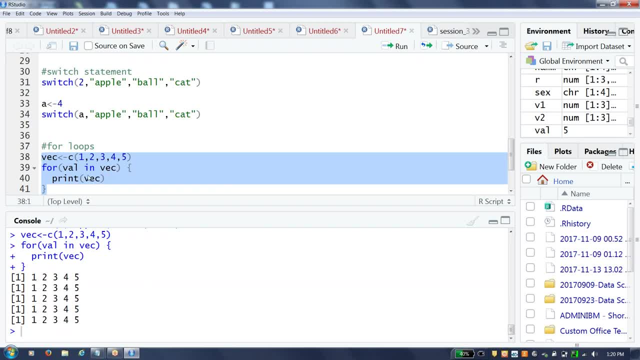 five, five elements. so it will loop for five times. so whatever the vector values we have here is going to print those, those actual effect. it will come first, initially, first one. it will come to loop first loop. and what is the? what are the values of vector we have here is 1, 2, 3, 4, 5. so it will print similarly a second time. 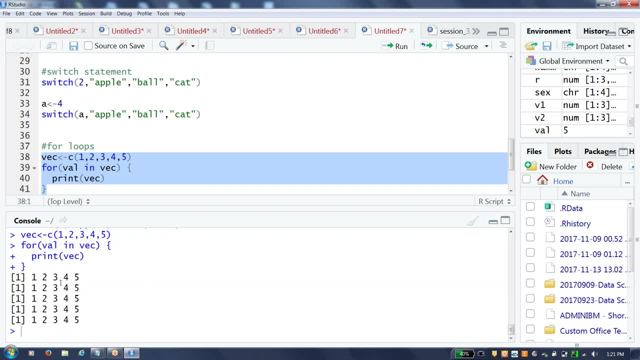 it will print effect: all vector, vector elements. third time, fourth time, fifth time, five times. it is printing vector values. so if I print instead of this, if I print value, so what is going to print is actual value of that loop. okay, so now we are looping for first time, first, second time value: value for V: L is to start. 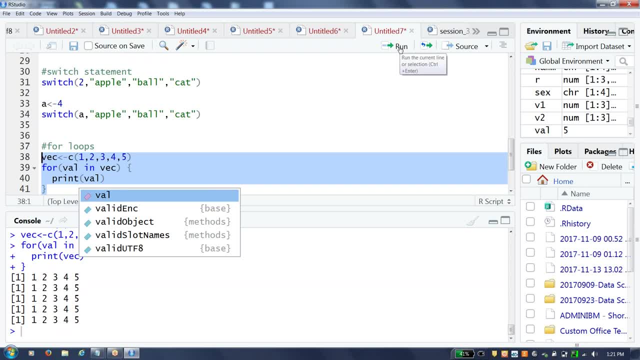 time V L for is 3, like that it is going to have. it is going to hold V L is going to hold the values 1, 2, 3, 4, 5. so that is what we are going to get here. so 1, 2, 3, 4, 5 is is going to take from B vector and every time 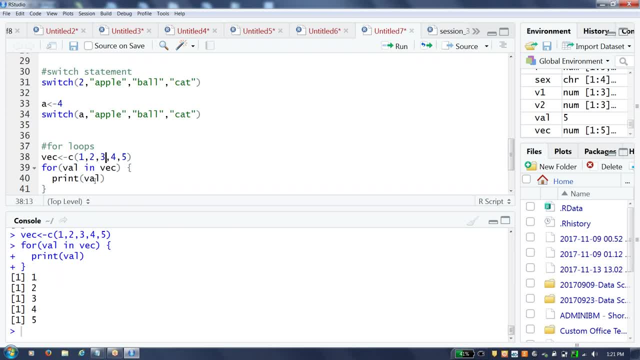 it is going to have other next element and that is what we are printing as a print: V L. so this is how that vectors- sorry for loops- is working. and let me go to next next end and break statements. suppose if I have the numbers like N, I have net 1, 2, 5, 5. 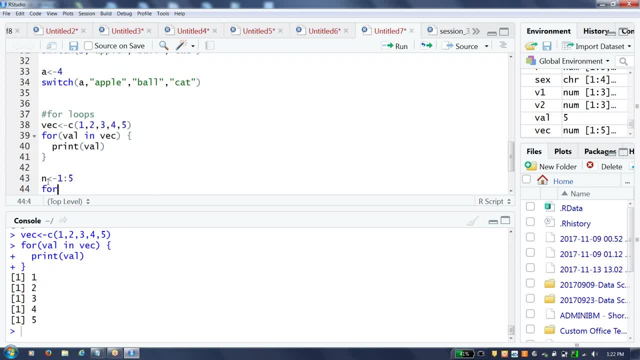 numbers I have. so same same thing I am going to do for I in N. so now I in all N values, one by one. we are going to have it in I. so what we are trying to do is I am going to use if condition here, if we I equal to, equal to 3, what I will do. 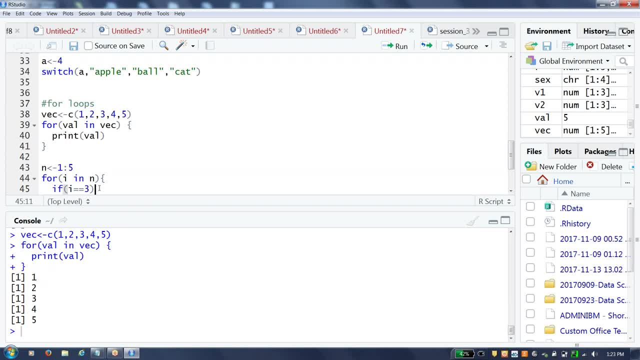 is, and to break this loop. I'm going to break this loop if, if that value is not 3, then what I am going to do is print, print I. so here I have five elements: 1, 2, 3, 4, 5 that are ascending N, so that five elements I am. 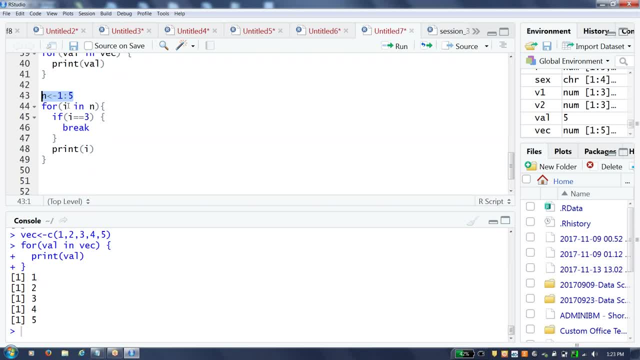 going to load it into I one by one. so first, if I will be having one, so it will check if I value is matching with three. no, it will not break. it will come to print statement, so it will print I, which is one, and then it will go back to. 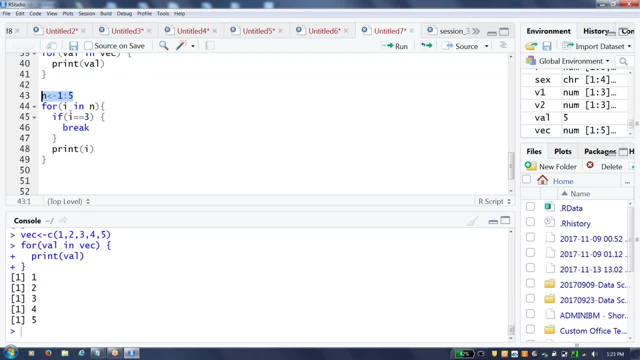 again. second loop: I is going to hold two and it will compare with three. so like that it will check. it is going to check this condition if condition it fails, so come to print and print the value 2 and then the I value of I is 3, so it will. 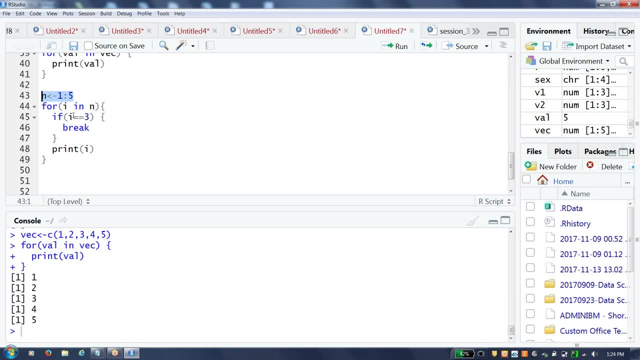 match I with 3, 3, so it will go a going go and exclude the each statement, which is break, so it will come out of that loop. so let me see what is going to happen here. break, so it is giving me the values 1 and 2. so because after, when it reaches to 3, I value 3 is going. 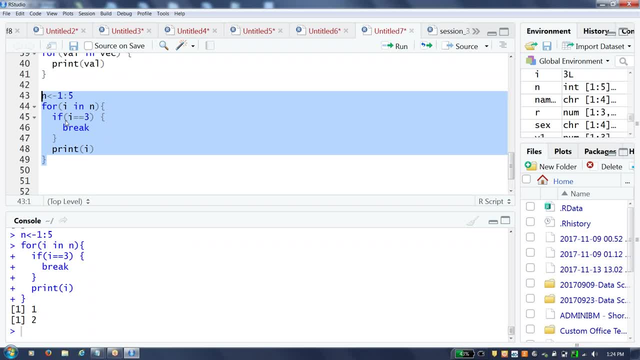 to match with 3. so and then it is excluding the break statement. so if condition is satisfied and inside if statement, we are telling the break so that it will come out of this loop, so it will not print any further, it will not exclude for any other value. so I am going. 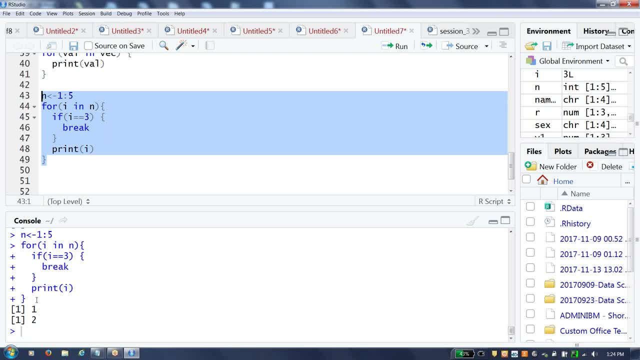 to print values in that for loop, 3, 4, 5. so simply, it will print only 1, 2. this is how break will work, so it will come out of that loop, whereas next statement, the same example, if I take it for next, what it is going to do is it is going to skip that value and it. 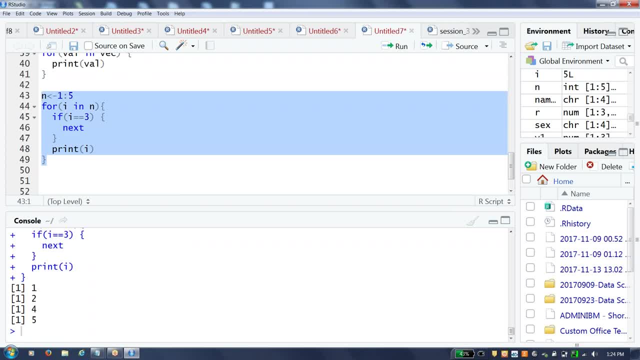 will. it is going to skip that value. whenever I value is 3, it is going for next loop, next iteration, which is third, fourth iteration and then fifth iteration, like that. so only when that condition matches that it is skipping. otherwise it is executing for all. so here: 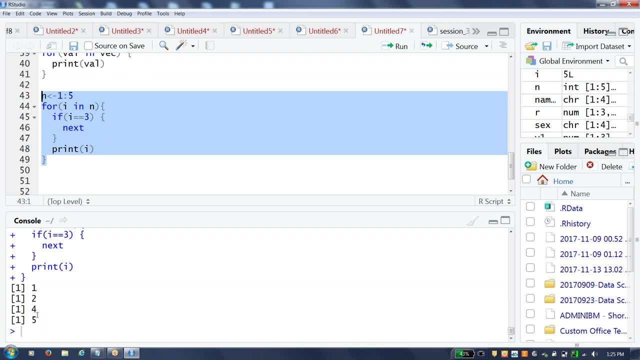 when you use next main, it is only skipping 3 and printing 1, 2, 4, 5 whenever it is break means it is breaking all, breaking the delant there itself. so that is the working functionality of this next 10 break statement. okay, so now we will move on to while loop. 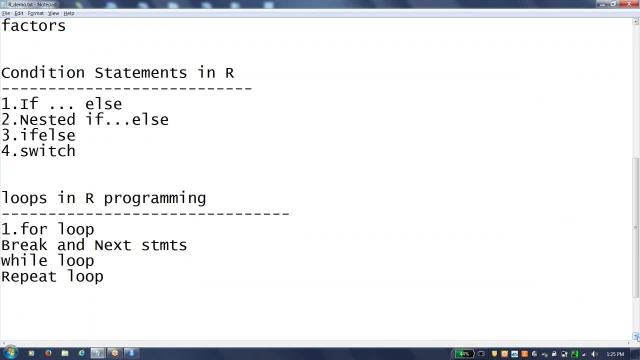 while loop is also a simple. it will check for a condition, while condition and what all statement we want to execute. we can execute and it will execute until that condition fails. okay, so while loop is like while some condition, if that condition is true, and it will go inside. 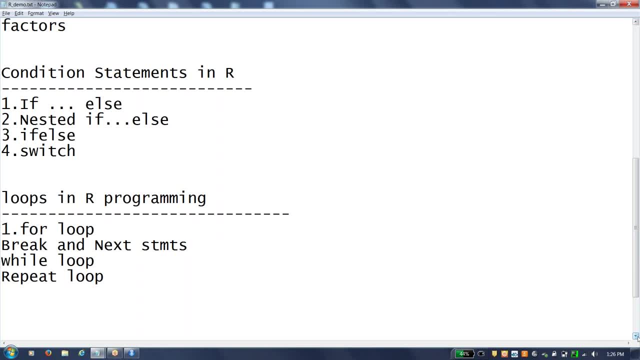 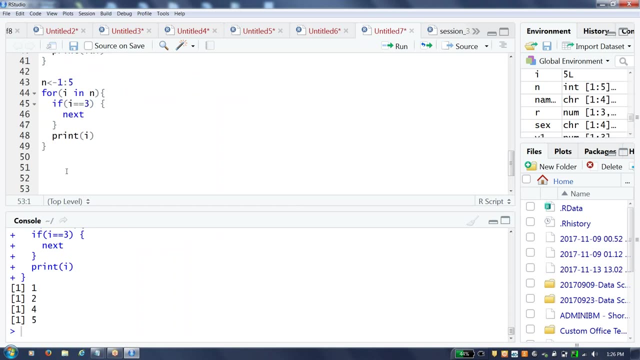 the loop and execute the statement. okay it like this. it will repeat until that while condition that condition is failed, so that that that also will not work. so now we are going to show you. I will show you example. it's just simple, very minimal, very basic basics. 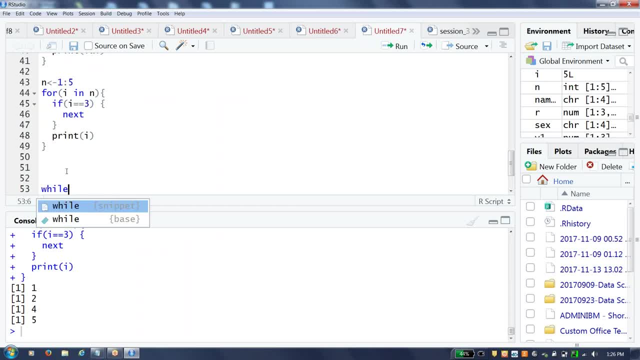 of any programming language. if we are clear here, then only we can go ahead with further actually, because we, if we don't know the basics here- it's a basics- then it is difficult to work on the further sessions actually, so that time giving here itself is simple things as. 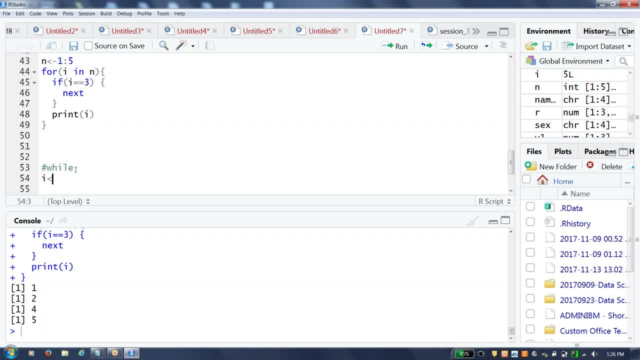 well, So while loop is like, I'm going to assign I with some value one, so I just simply have I value one. so what I'm going to do is, while I less than six is six, less than six, what I'm say print I am going to print I, so I'm going to increment it. okay, it's. 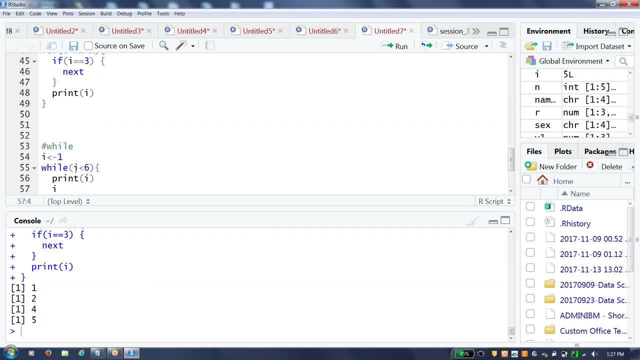 known, known fact: only some tail increment. I equal to I plus one. so how it works is like it. it will, first I value will be one, one is less than six, true, so this condition is satisfied. so it will go inside the loop and print to the value I is one, and then and then what it will do is it will increment. so 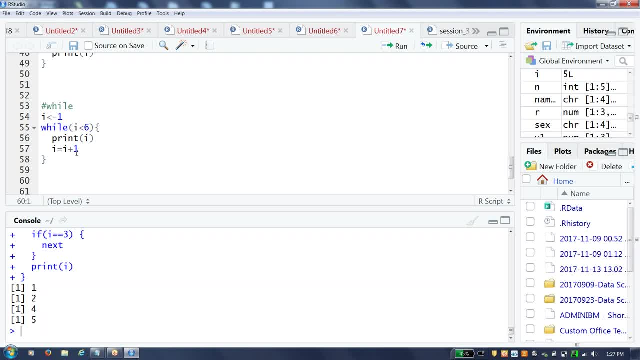 to I value become to two less than six. it will again print and increment three, three less than six. four print four. four less than six. print five. five less than six print and then six condition is going to fail. six less not is six is not going to be less. that's not six is not. 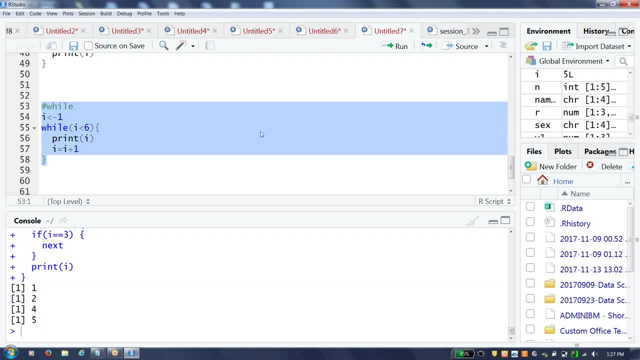 less than six. so the condition is failed and it's going to exit that loop. so this now will statement is going to work in. our programming is like it's a similar to any other programming. so explain: it is printing one to five numbers, the last one which is: 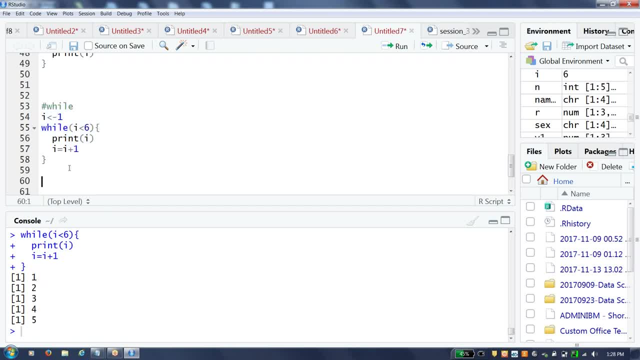 I am going to explain here is that repeat loops. so we put repeat loop things like repeat this is like do well, only so, first it will do and we are going to mention inside the break statement when we would like to break this and otherwise it will keep on repeating on it. so same same, same way. I. 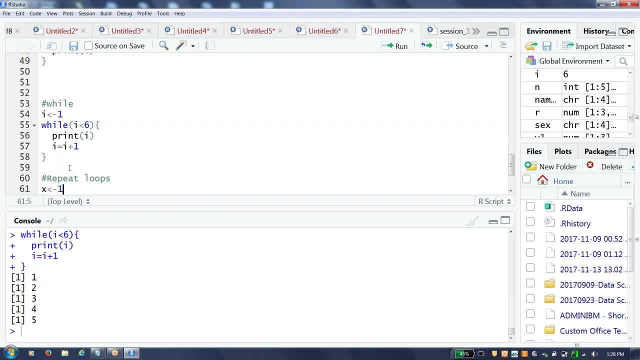 can write same kind of logic xx. I'm going to ask the first, initially one, and then repeat: is a keyword the keyword, and what I'm going to do is print I, printing I initially as a print X. the initial X value is one, so it will print X. so then what I will do is: 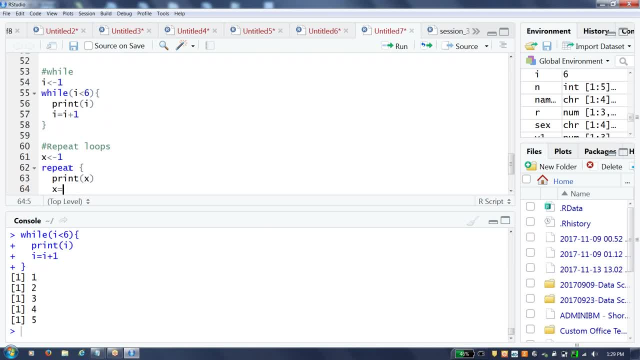 I will increment this, so x equal to x plus 1. okay, I am going to increment this one. then what I am going to do is I am going to write an exit statement, otherwise it will go infinite to 1, 2, 3, 4, 4, 5, info till infinite, till never exit. if I didn't. 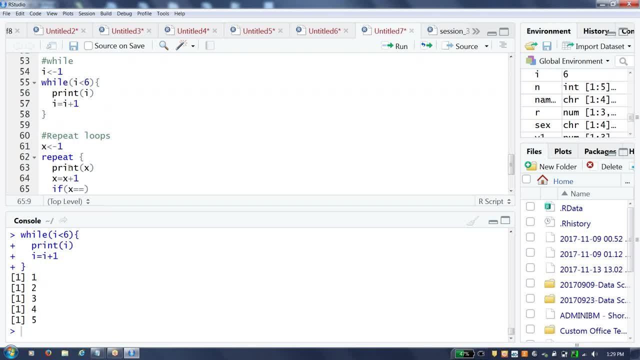 think, then exit condition in this repeat loops: okay. so what I am going to write is: exit when, if, if x equal to equal to 6. what I am going to do is that I will throw quick Drive. what I'm going to say: who says break, that's it. so it is going to end that a. 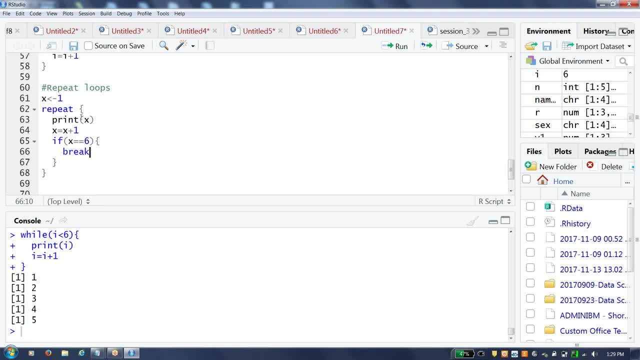 repeat loop. so it will print first initially one, then it will increment to, then will print three, four, five, and then it will, whenever that increment is happened, six, six, then it will check the condition six, so six itself it is breaking. it is not going to print the six. so whenever the five is printed, then 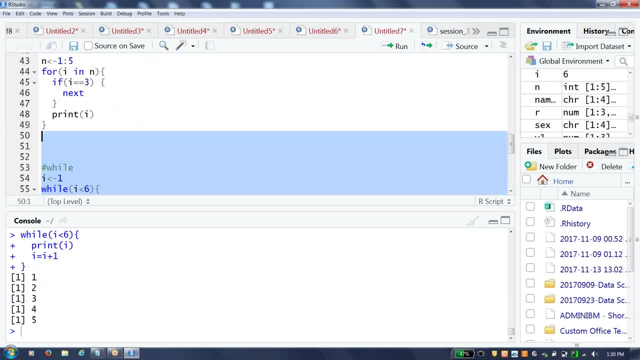 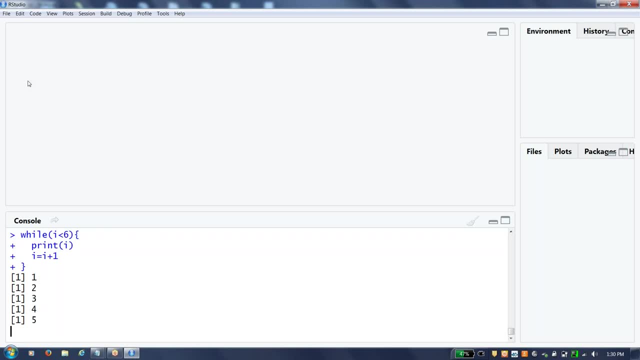 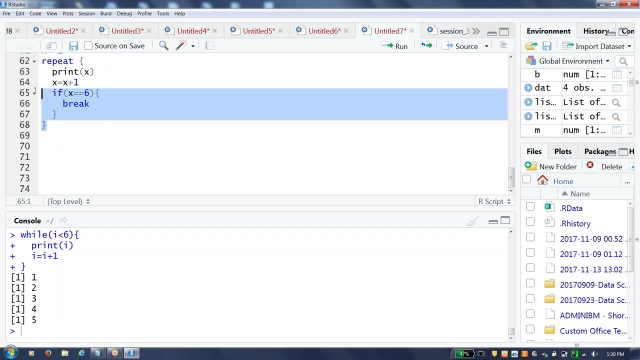 it is incremented, then it is checked for the condition. condition is failed so it is going to exit that loop. so let me exclude this one repeat. so one, two, three, four, five. so this how this repeats loops also work. so in next state, next video, I am going to cover some basic. 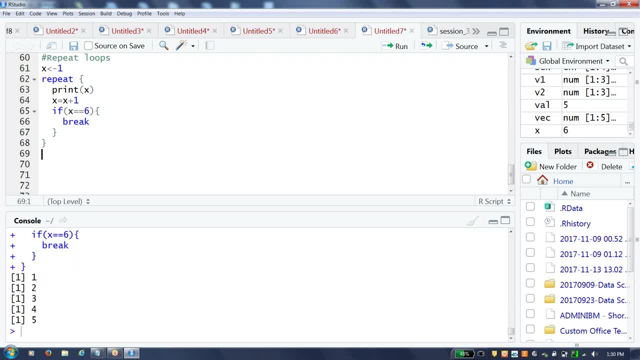 functions which we are using in our programming. so then, after that, I am going to explain how to create our own user defined functions. likewise, I am going to continue. so, so this, this is what I would like to cover in this video about conditional statements and loops. okay, okay, thanks for watching, please do. 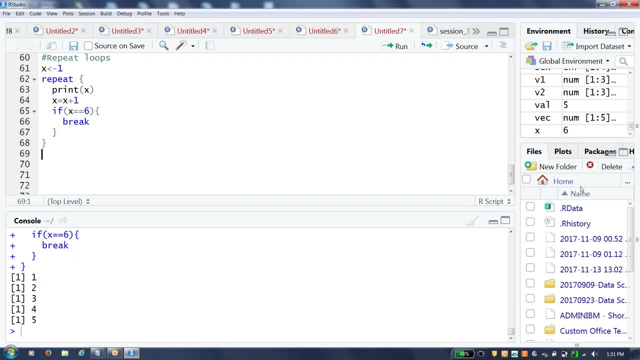 like and subscribe for more videos. thank you.